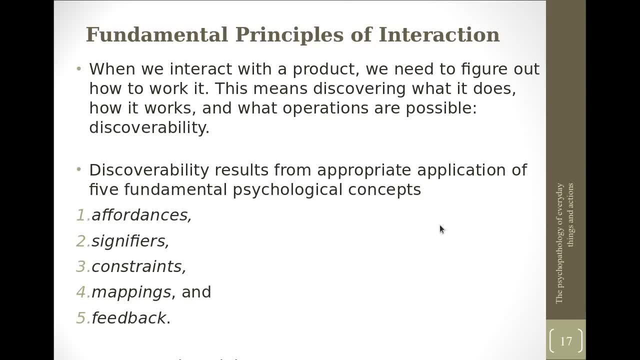 Welcome to this lecture. Today we will see the fundamental principles of interaction. Now, what are those principles? To know this, let's understand: when we interact with a product, we need to figure out how it works, how to handle that, how rather it basically is being 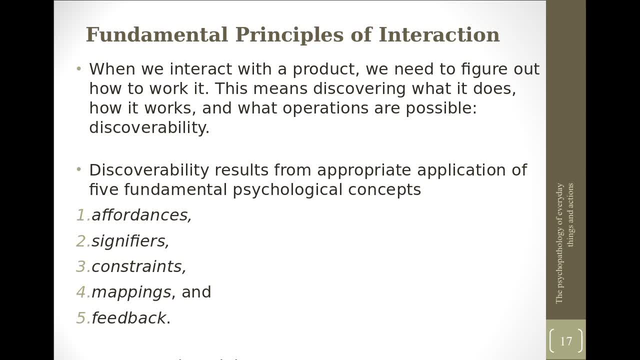 operated. Rather, this means identifying, discovering what it does, how it works and what operations are possible with it. That is what is called as the discoverability. Now, the discoverability results from the appropriate application of five fundamental psychological concepts, which are basically called as the fundamental principles of interaction. So 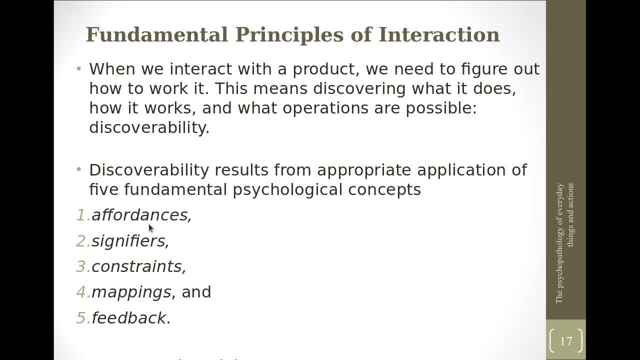 these are as follows: The affordances, signifiers, constraints, mappings, and the last is feedback. There is also one principle which is rather to be understood only when, in exam, you have to write these five. So that is also called as the conceptual model. 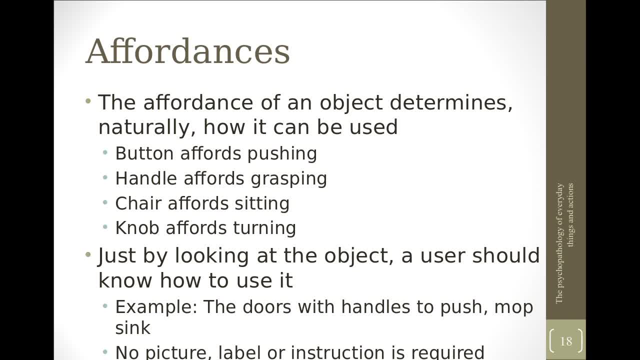 You will see that The first is affordances. Now the singular word here is affordance Rather. that means the affordance of an object determines naturally how it can be used, So what operations are possible with it. for example, we can say: So that is what is called as the affordance of that object. So for example, 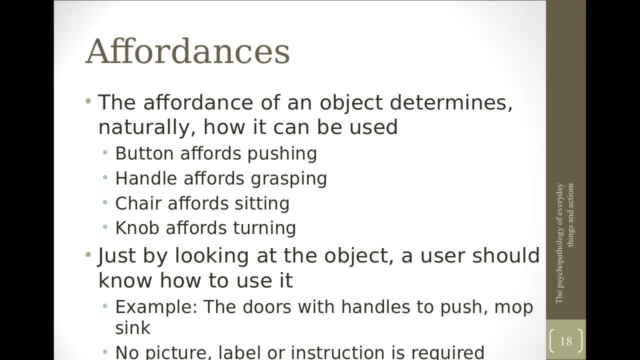 button affords pushing A button, if it is there that will allow us to push it. Handle affords grasping A chair affords sitting on it. A knob affords turning it. So these are the various affordances of that particular object. 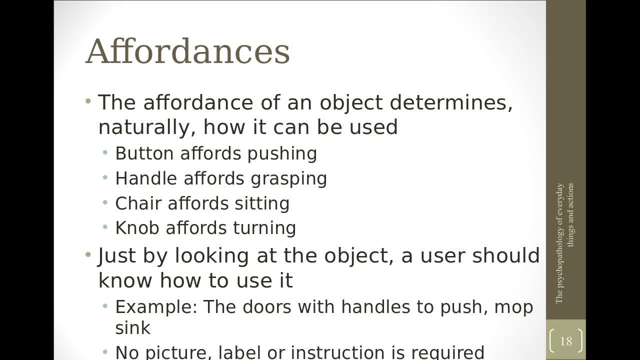 Now, simply by looking at the object, a user should be able to know how to use it. That is what is very important so far as the interaction design is concerned. The affordance of any object must be very much clear, So previously we have seen the doors with handles to push. 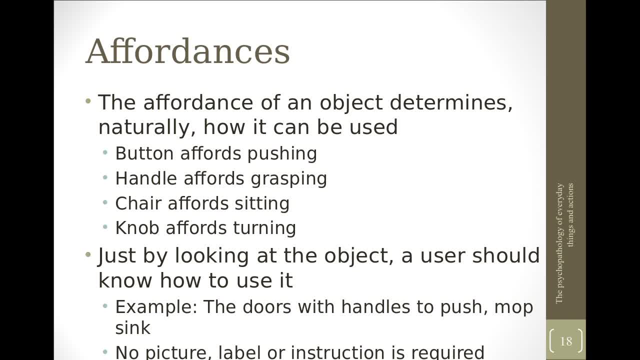 So it must be clearly understood by the user whether to push that door or pull that door off. No extra instructions or picture or label is required to know how to operate. that If the instructions are required, for some notations or pictures are required. the affordance. 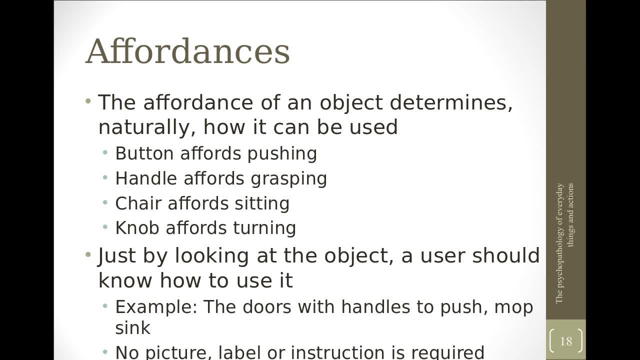 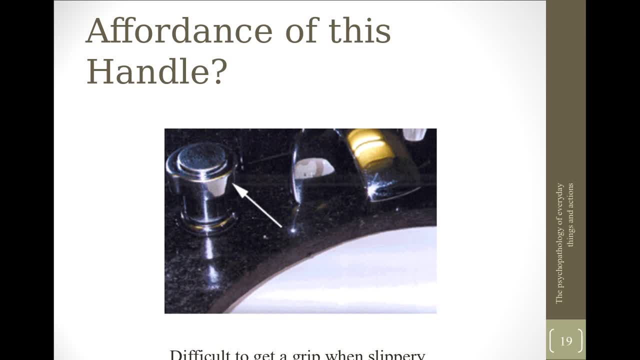 is not that clear. So, for simple affordances, extra information should not be required. Now to know what is the affordance of this handle, if you see the picture, Well, it is seen that it can be tilted, But it will get slippery when it is wet. 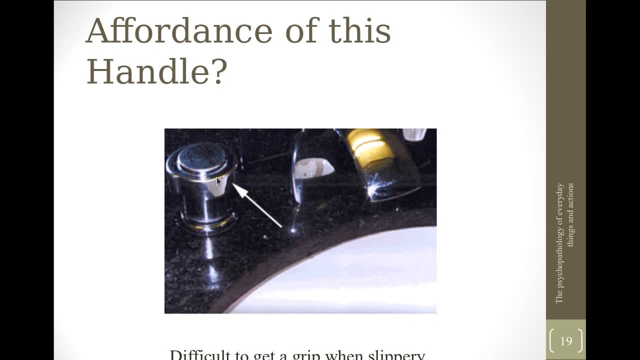 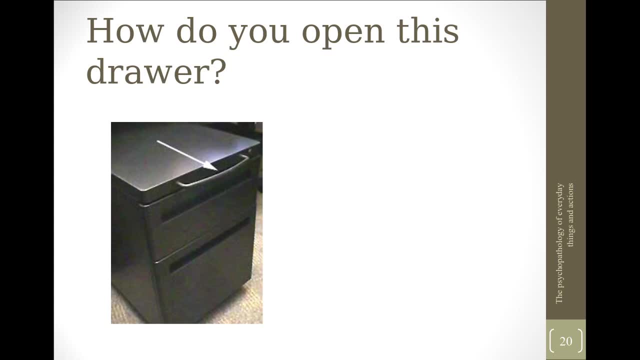 For example, because of the glossy nature of that handle, that may be slippery. Now, if you see this picture, there is a cupboard, small cupboard, which is having a handle there. Now how to open the drawer beneath with that handle or not? 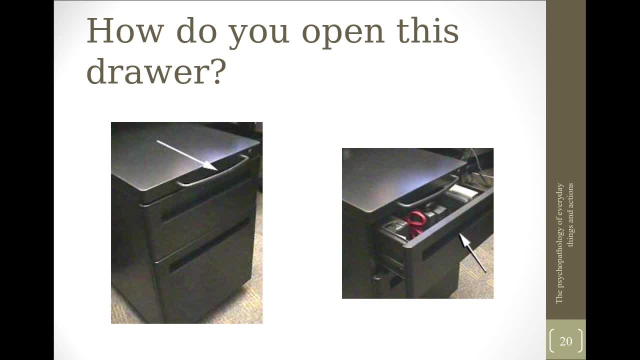 It appears that the handle is not to be used while opening the drawer, So there is a separate groove for that which is to be used. So the affordance is not that clear or confusing. you can say The control here is not that clear and it is not clear how to use this. 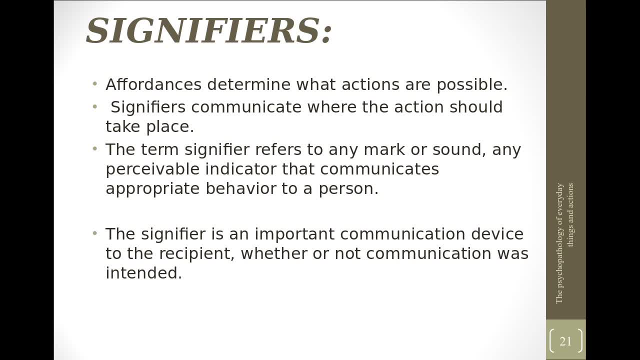 Next is signifiers. Now we have seen that affordances determine what actions are possible. Now signifiers: on the other hand, they communicate where the action should take place. The term signifier refers to any mark or sound, any perceivable indicator that communicates. 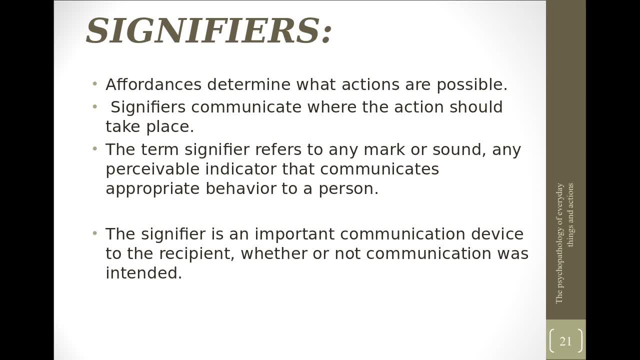 or tells appropriate behavior to a person. The signifier is an important communication device to the recipient, the user. you can say whether or not communication was intended. That means it has to be there, even though sometimes communication is not expected. It's a communication, a very important communication pattern, communication device so far as the user is concerned. 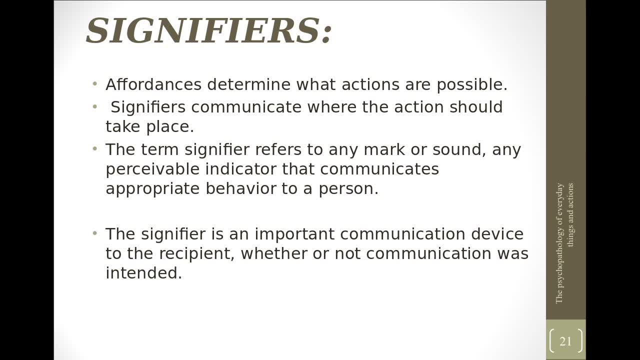 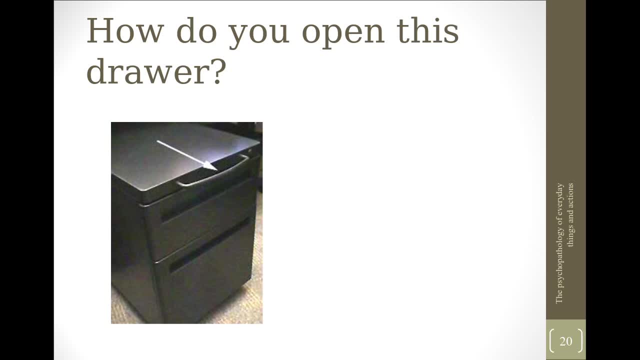 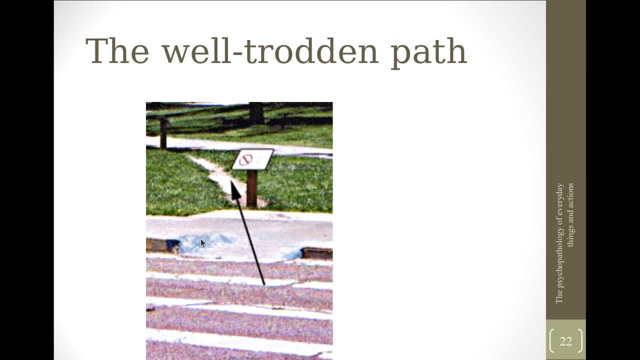 Previously. you have seen that In the drawer example it was not clear what the handler was doing, whether it was there to open the drawer or not. So signifier has to be there. We'll see with one example Now. in this picture there is a path, a road, you can say, where there are some objects to be preserved besides it. 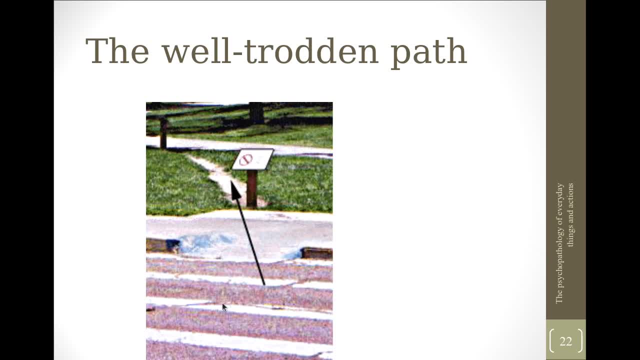 So that may be. you can say: any garden where it is not expected that people walk over those objects, The landscape preservation site it may be, for example. So there is one signifier: a board you can say: please use sidewalks. 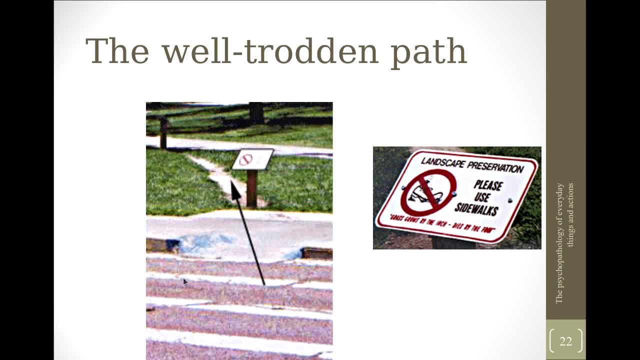 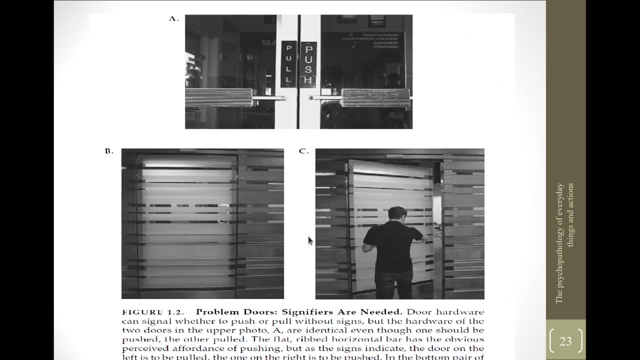 So people may walk on this. to prevent that, There's a signifier that tells We should not, or the people should not, walk over this way, rather on this sidewalks. Now, here the signifiers are required. If you see, There are two doors in figure A. 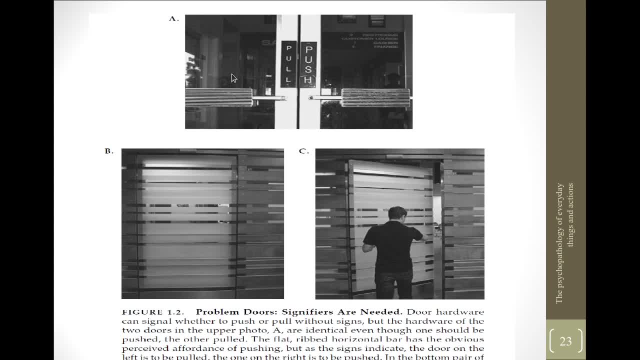 One, the left, is to be pulled, whereas the right is to be pushed, Even though both of them are having the handles Which rather call for pulling them. So for left it is okay, For right it may not be okay. 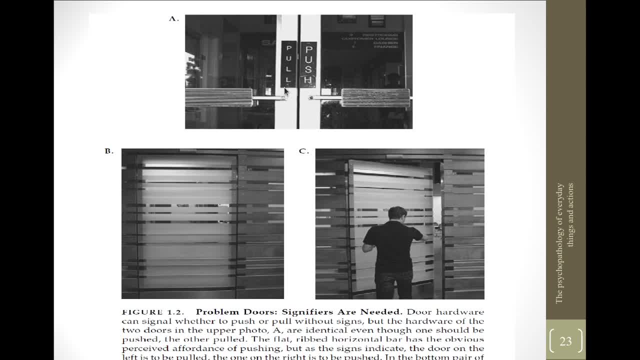 So the signifiers are required. What is to be done for what door? Here? on figure B and C, if you see The door, is there a glass door Where it is not clear that, whether it opens at its left side or right side. 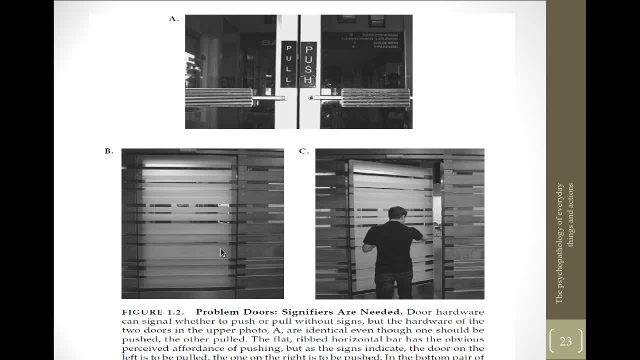 That may be a confusion. The user may have to Go with trial and error. So there are no visible signifiers you can say, Because there are no even handles Which tell where, which part or which side the door is to be opened with. 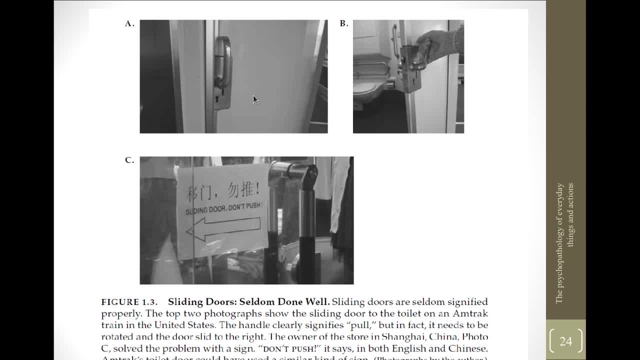 Now, if you see The toilet door is shown here, Where it appears with that handle, It sounds that it appears that it is to be pulled off, But rather in practice it is to be slided. So this problem is taken care by having a label fixed to the glass door. 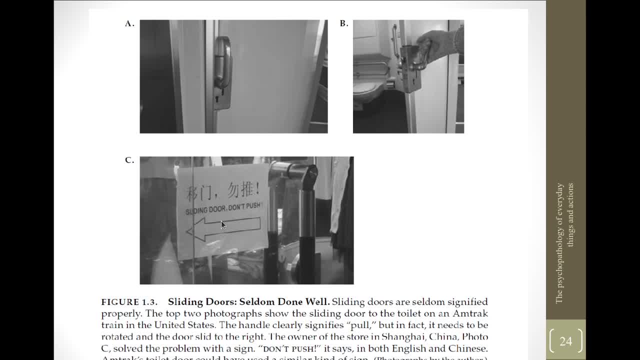 On the third diagram or third photo, you can say: Where an explicit indication of the door to be slided is given, Do not push Slide the door That is given. So if that is required to be put, The design is imperfect. we can say: 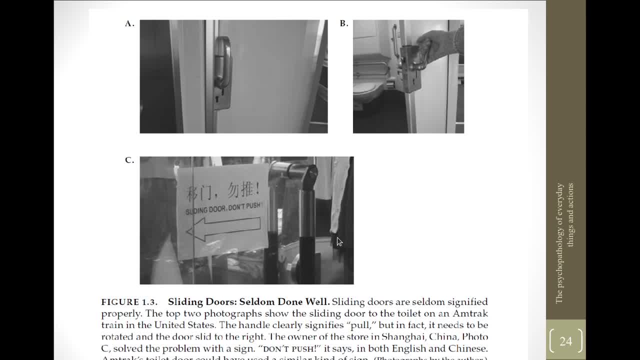 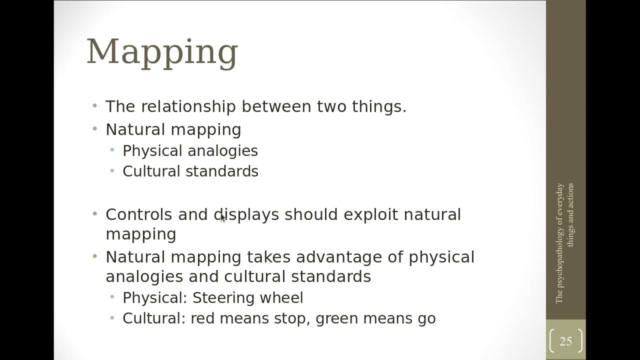 So You have seen why signifiers are required. When the interaction is not clear, We may require to give extra information Of how to handle that, And that is what is called as the signifier. The third is mapping. It rather means the relationship between two things. 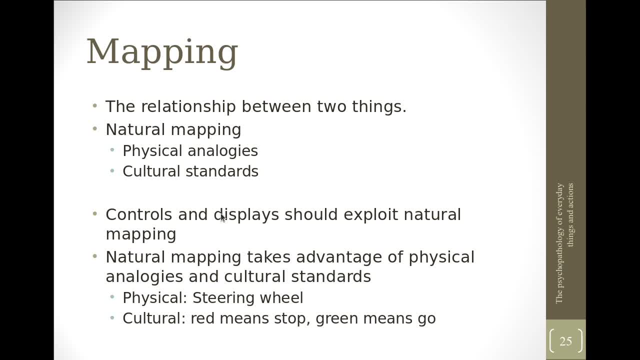 Or the natural relationship between two things. So there may be natural mapping Because of two things: One is called as physical analogies And second is cultural standards. We will see that with examples, Now the controls that we design for any interaction or any interface. 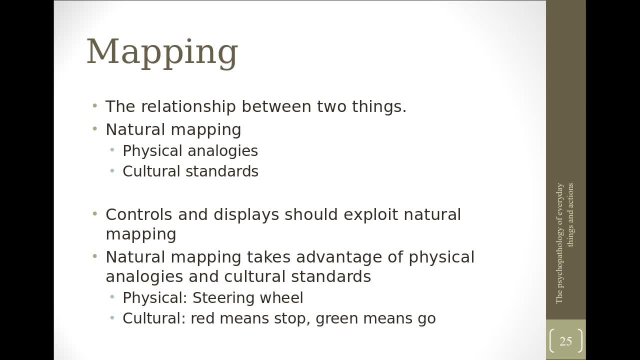 We can say UI, Or it may be a display. They should exploit the natural mapping. What is that? We will see with one example. Now, natural mapping takes advantage of physical analogies and cultural standards. Now, what is that natural mapping? What is that cultural standards? 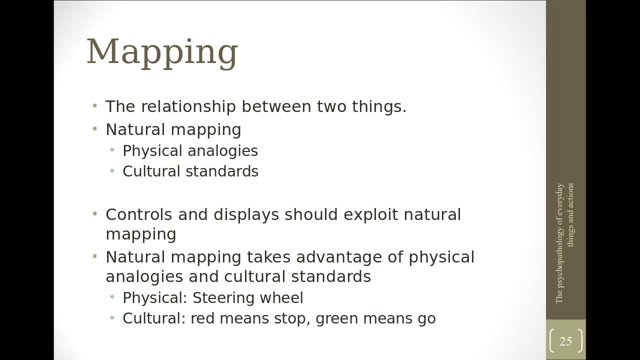 We will see. So far as the physical analogies or mapping it is concerned, You take one example of steering wheel To turn a car towards right. There is a steering wheel Which is to be tilted in clockwise direction, Indicating the car is to be tilted or turned towards right. 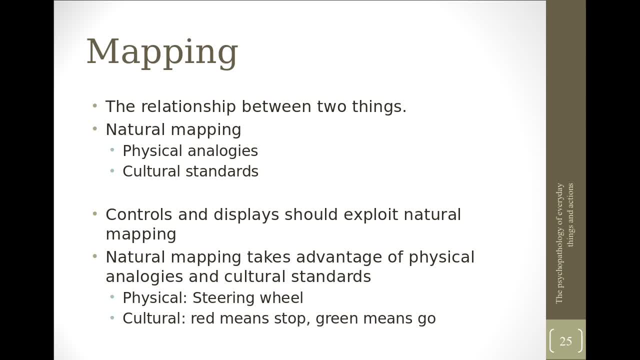 That's a natural mapping. We turn the steering towards right In the clockwise direction, And the car gets turned towards right. Oppositely, if you turn towards left, The car will turn accordingly, Proportionately towards left, And there are cultural mappings as well. 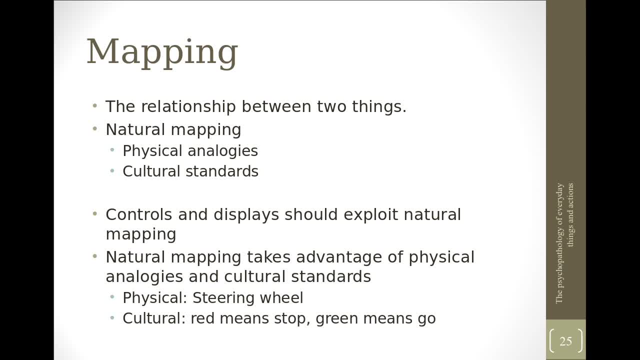 Well, culturally, mostly throughout the globe, Red indicates some kind of problem, Danger, And that means, for example, If a button is there with red color, That means if a problem is there, It can be used to stop that device, Whereas green means to go. 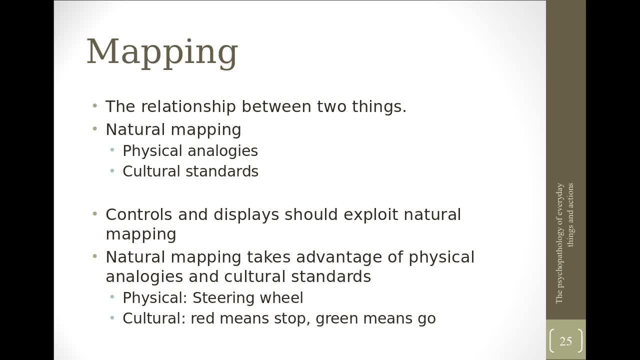 Green indicates success. That means if you want to start that device, If you want to go further, That can be green. So that's a cultural mapping And whereas we have previously seen The physical mapping of In the example of steering wheel, 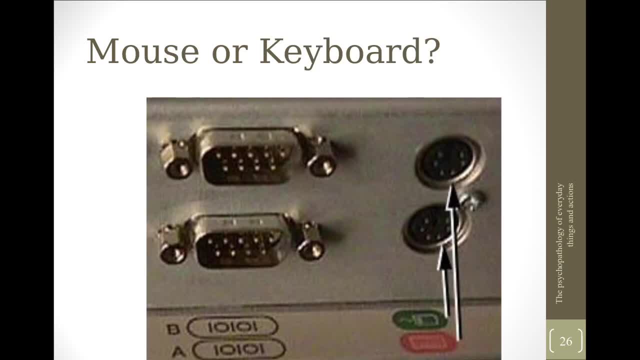 So this diagram indicates, or the picture indicates, The back of CPU, Where there are two ports, One for keyboard, One for mouse, Where it is not very much clear Which is for what, Whether this is for keyboard Or this is for keyboard. 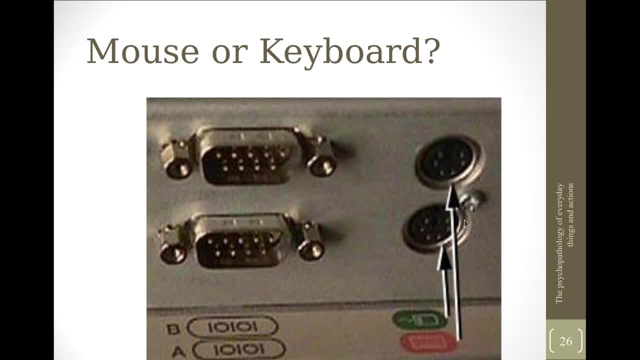 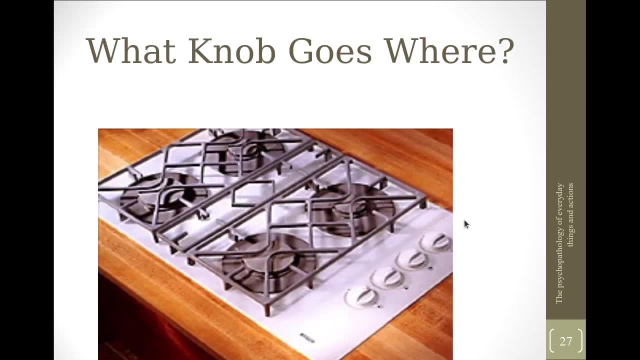 Or this is for mouse, Or this is for mouse. So you might have seen in the Some other examples There are different colors used, One for keyboard, One for mouse. Now, This is a gas stove Having four, I mean. 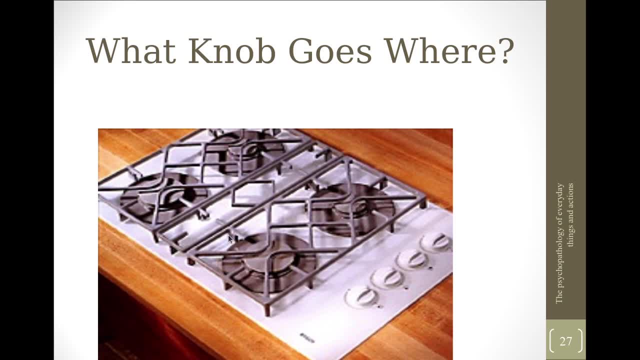 Four stoves And there are four knobs, Each of Each for one stove, But it is not very much clear Which knob Is for which stove. So if you, If you are having one example, Let me check that. Yes. 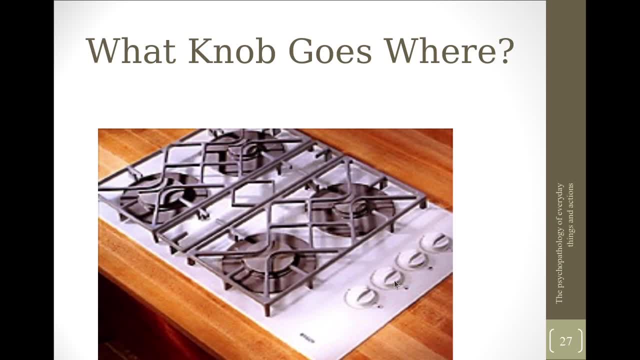 It is not here, Had that been the case, that The four Knobs were arranged In the same fashion As The stoves are there. They were of The same Pattern here, In that order, In a rectangular fashion. 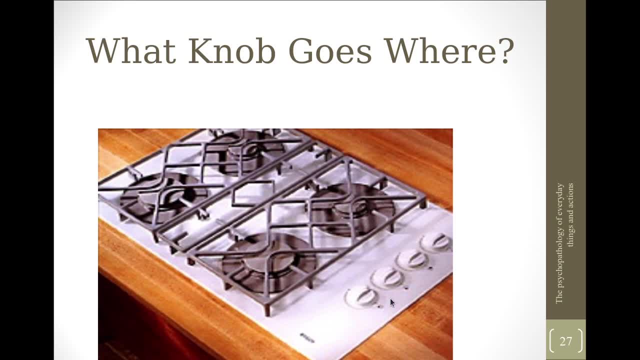 It would have been Very much clear Which knob Controls Which stove. That's a Natural Or Physical Mapping. You can say This is what is called as mapping: We know Which controls Which stoves. 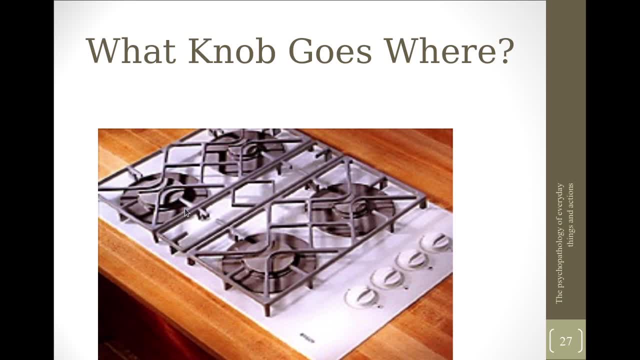 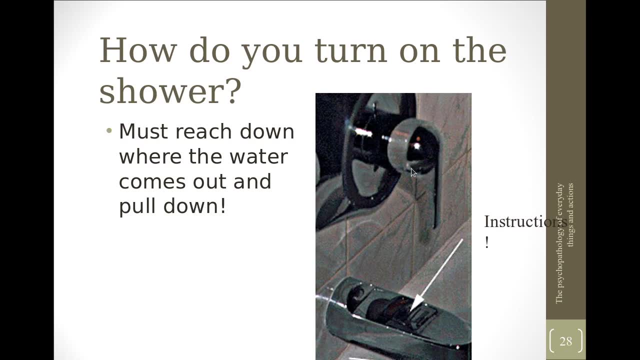 Which control Is used for Which particular Part of that Interface Or that device. Now it is In the case of this shower. How do you turn on the shower? So the If there are some Instructions Required. 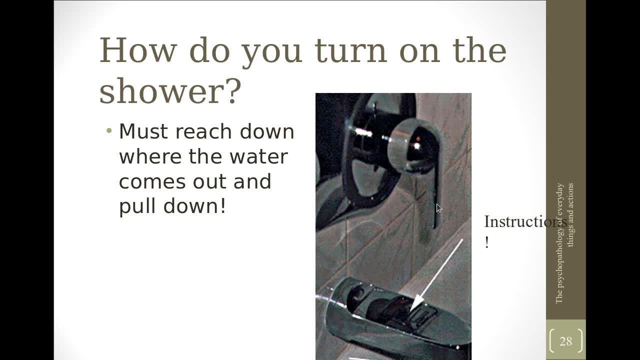 To be given That Mapping Is not That Properly Utilized Here. You must Reach Down Where The water Comes out, And It Comes Out And Pull It Down. 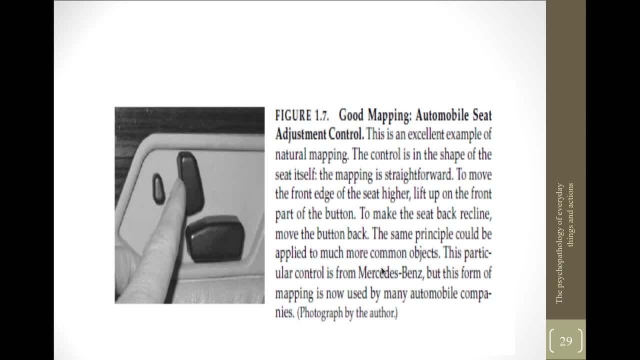 One Example, Once Again, Of Good Mapping. Here An Automobile Seat Adjustment Control Is Shown, Which Is Exactly In The Shape Of The Seat You. 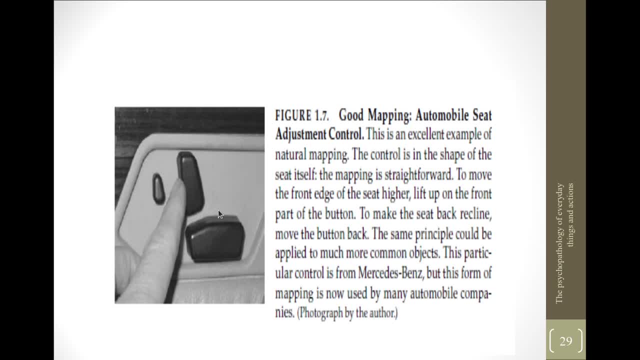 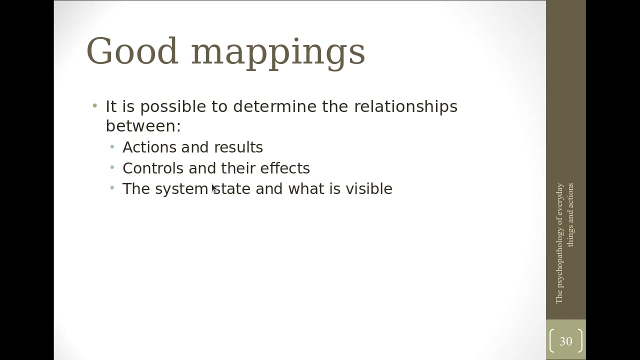 Can Simply Control That With This Knob. You Can Put It, Pull It Up So That The Seat Gets Higher. You Can Tilt It Forward. 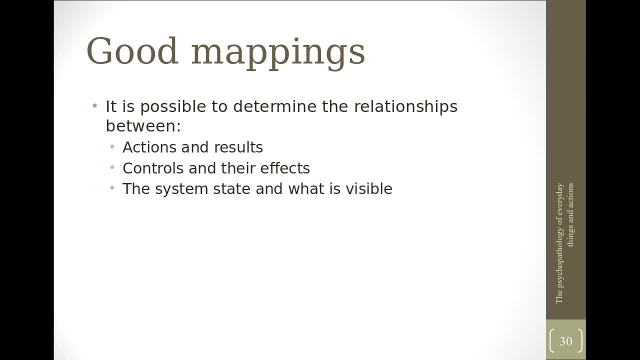 Or Backwards In The Actions And The Results. If You Tilt The Knob Towards, I Mean Forward, Towards Front- The Seat Will Get Aligned. 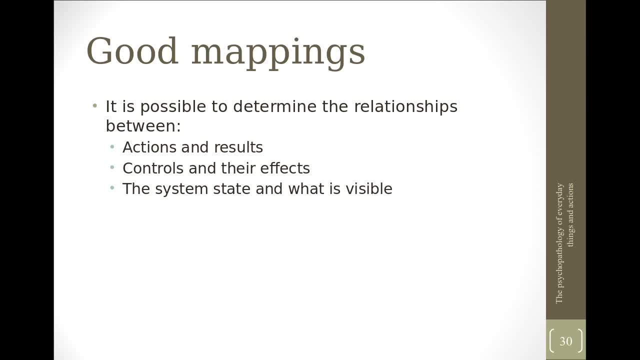 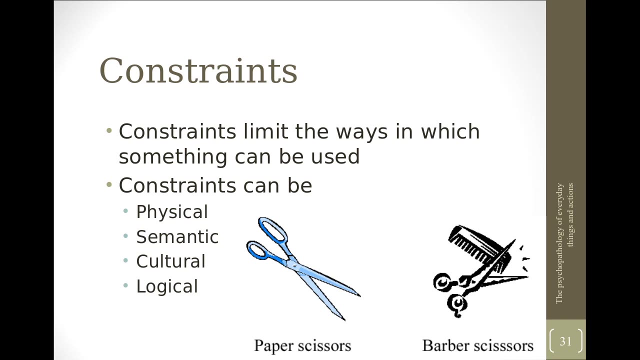 Accordingly, The Back Of The Seat Will Tilt And The System State. And What Is Visible. That Is Also Clear. The Next Is Constraints. Now 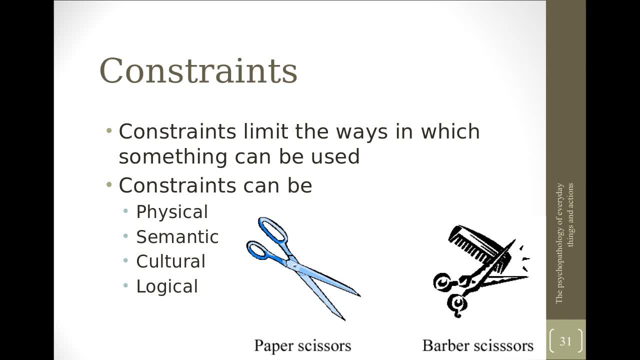 Constraints Limit The Ways In Which Something Can Be Used Now Other Usages. We Have To Provide Some Constraints, So Constraints Can Be Physical. They 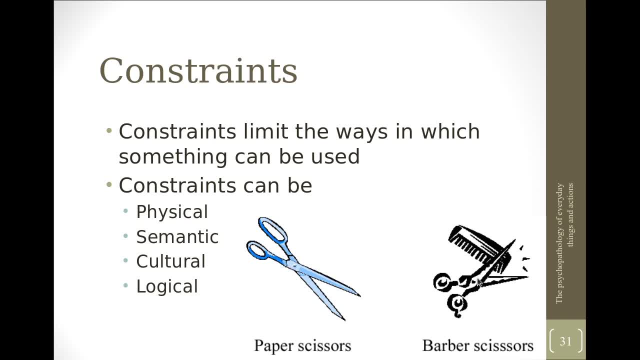 Can Be Semantic, They Can Be Cultural Or They Can Even Be Logical. Here The This Way, Whereas The Barber Scissors Are Designed Well, The 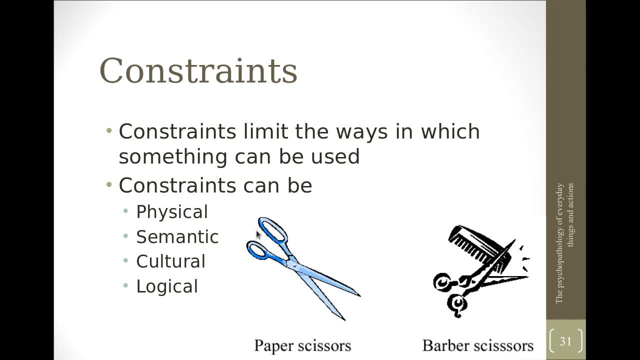 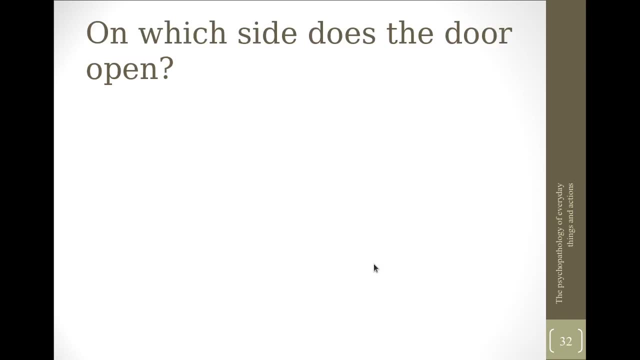 Paper Scissors, I Mean They Optimally. They Can Be Used With Any Finger In Any Part Of That Scissors. Well, Here On Which Side. 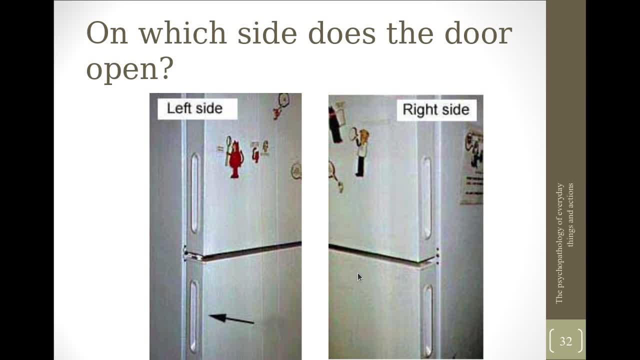 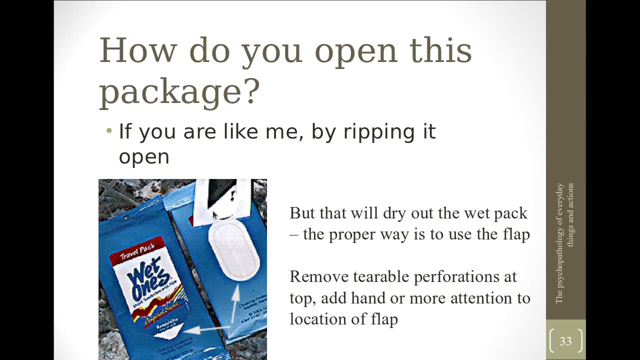 Does The Door Open Left Side Or Right Side? That Is Not Clear. So If We Are To Open The Door On A Specific Side, It 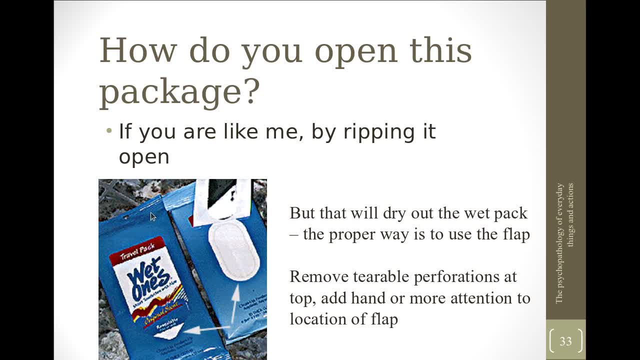 May Appear That Well, The Upper Part Can Be Turn Off By Ripping It Open, But If That Is Done, That May Dry Out The 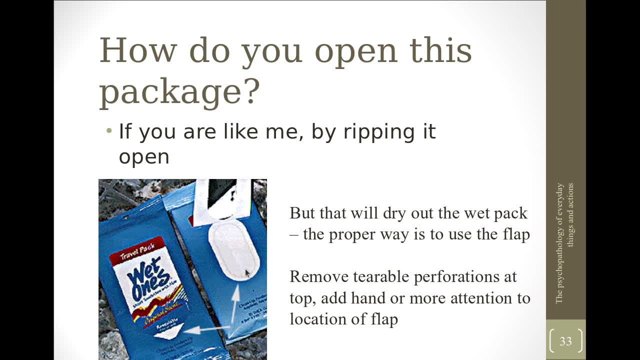 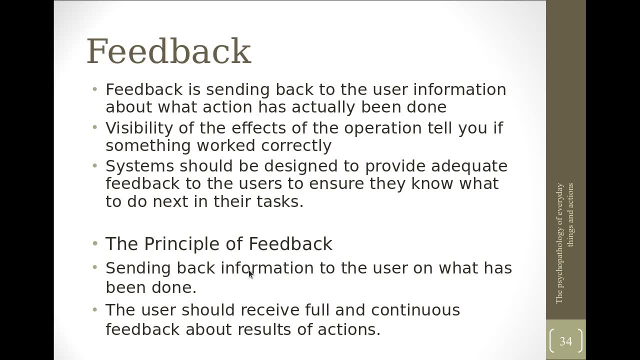 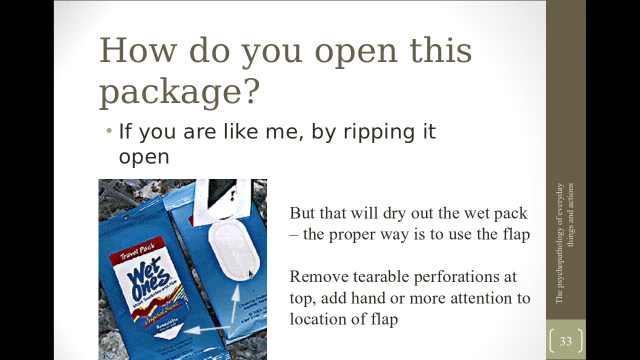 Weight Papers Inside. The Door Is Open. That Is Clear. Now We Have To Open The Door And Open The Door Is Open. Now We Have 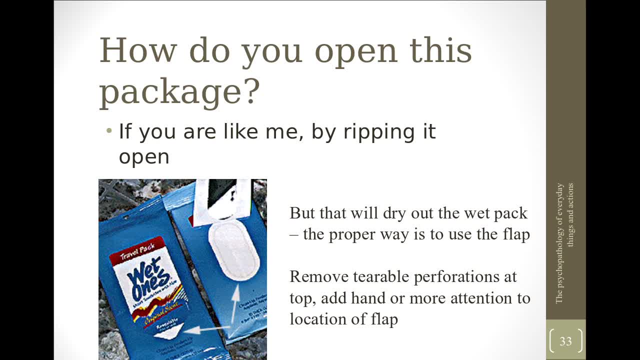 To Open The Door And Open The Door Is Open, The Door We Have To Open. The Door Is Tilted And Can Be Tilted. 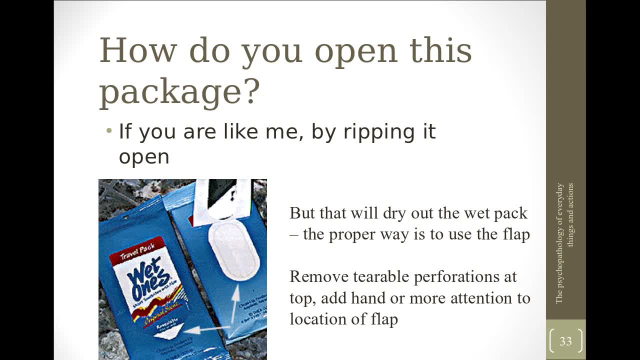 That Is Open. Now, That Is Open. A Door Is Open any specific direction. so a constraint: if it is to be provided, say, for example, for a knob which is can be rotated only in single direction, explicit arrows are required. that is not a constraint, that's a signifier. 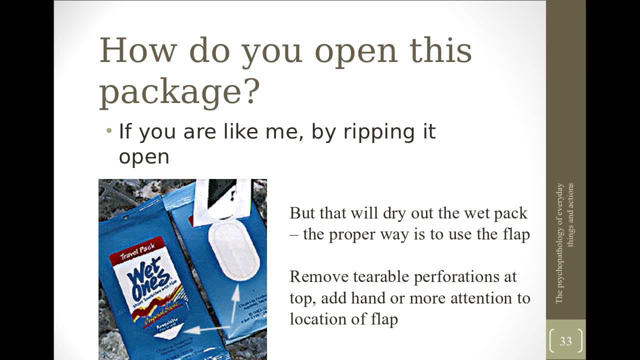 so, otherwise people will see and think that has to be tilted in both the ways, from left to right, right to left in the. on the contrary, in the case of a button, a push button, that can only be pressed, that can cannot be rotated. so next is feedback. feedback is sending back to the user. 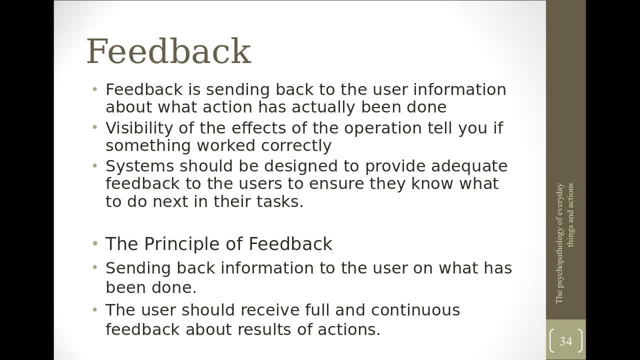 some information about what actions has actually been done on the UI or by the device. you can say visibility of the effects of the operation. they tell the user if some something worked correctly or not. for example, if we press a button and the button appears to be pressed because of the change in the design, that may on the screen. i am saying that may. 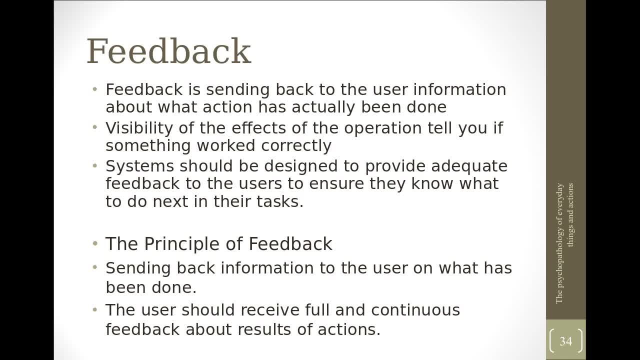 say that the action has started, for example, if there is a sound that may even give the feedback. now, that's why system should be designed to provide adequate feedback to the users, so as to ensure them that what the next action will be done, that operation will be done, that will be given to them. 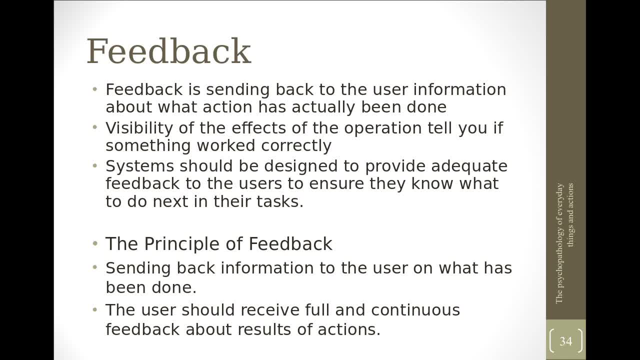 Now the principle of feedback: sending back information to the user on what has been done. that is the main purpose or principle of the feedback. the intention here is that the user should receive full and continuous feedback about results of actions. it's not sufficient. 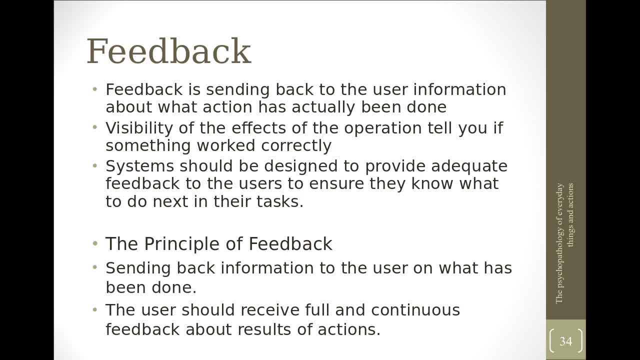 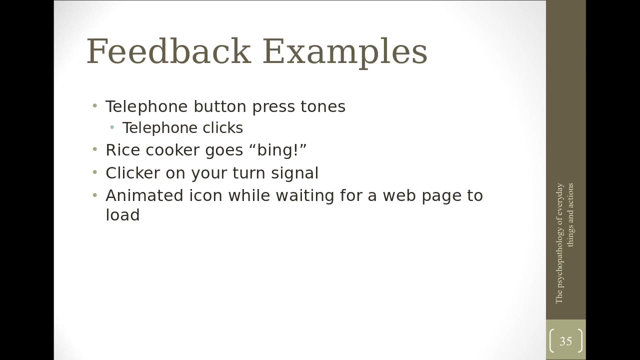 that if an action is having some duration, you should continue to provide the feedback over time. for example, if the file is being downloaded, the continuous percentage of how much percentage of the file is being downloaded has to be displayed. so there may be one example. 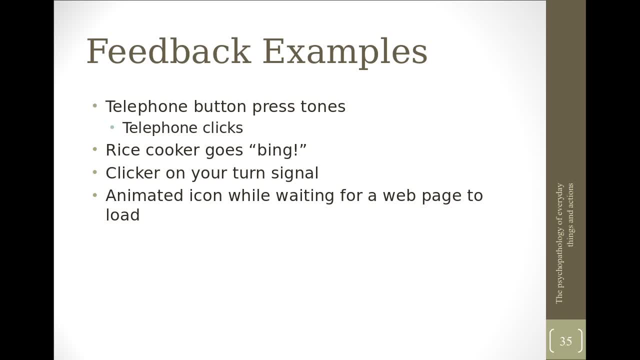 of telephone button press tones. that's an event: we press a button and there is a sound that indicates that the button has been pressed. Now, when the cooker is opened, I mean it goes with that bing, so it will make that sound when the appropriate temperature. 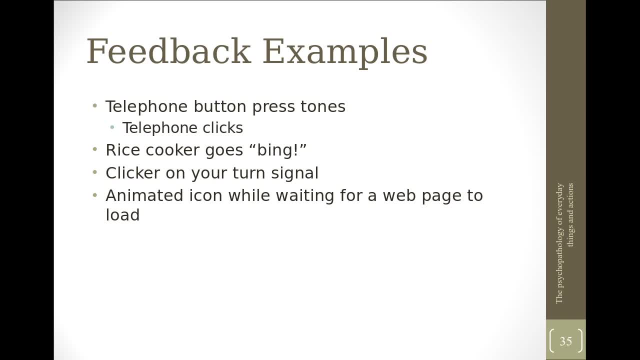 is reached, for example, the cooking is done. so if you consider the turn signal of a vehicle, it will indicate one sound. while the web page is being loaded, there may be an animated icon that indicates the sound, So you might have seen that. so these are the feedbacks. they indicate that the operation 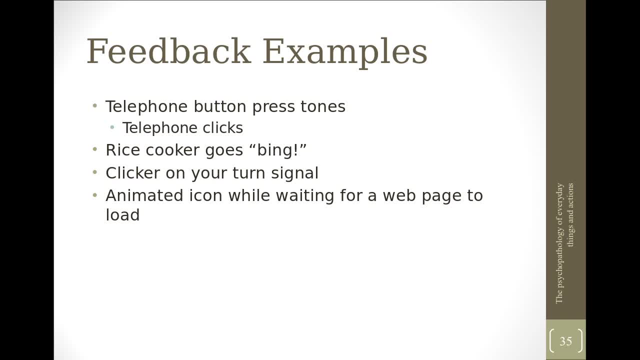 is being done otherwise had there been no feedback. for example, as we have discussed previously, we enter a command which may take some time to execute and the prompt does not display anything. we are simply not knowing whether the system is working, is processing. 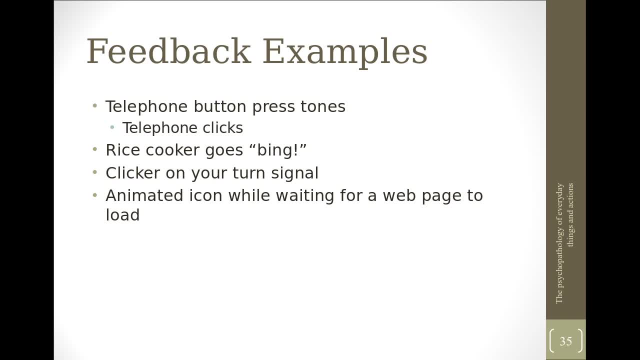 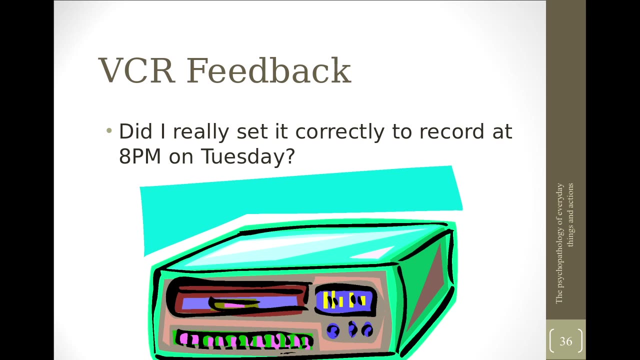 that thing or not, The system is hanged. the system is something, for example, is not functioning properly, so that may not be clear and that's why some sort of feedback is necessary. One example is: once a year a VCR is shown where some timely recording is set. but if 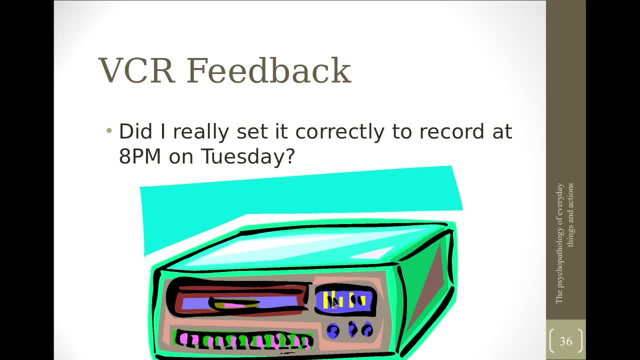 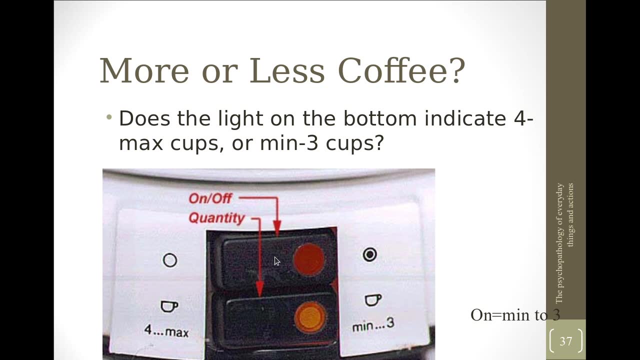 that indication is not there on the screen. the user is not sure whether the recording was set on a particular screen, So the VCR is set on a particular time and day. In this coffee maker here there is one on-off button and the proportion: how much cups of? 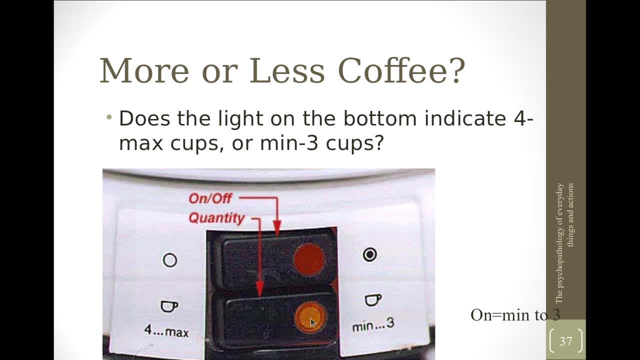 the coffee is. there are two indicators here, so one for minimum 3, for maximum 4.. So what is that light indicating on the bottom? It indicates maximum Maximum 4 cups or minimum 3 cups. that may not be very much clear. 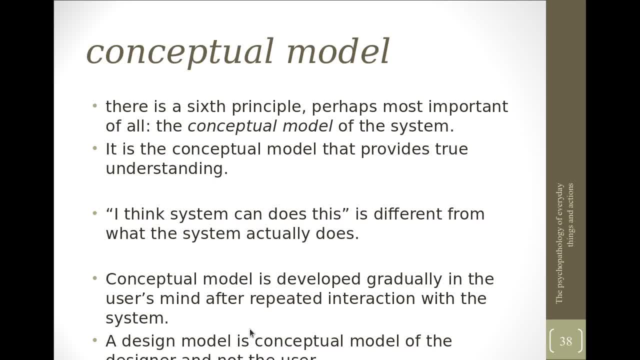 And, lastly, whether it is- I mean, actually it is not to be- written in the exam, but we will see that that is what is called as the conceptual model. There is a sixth principle that may be, or that is perhaps, the most important, that is: 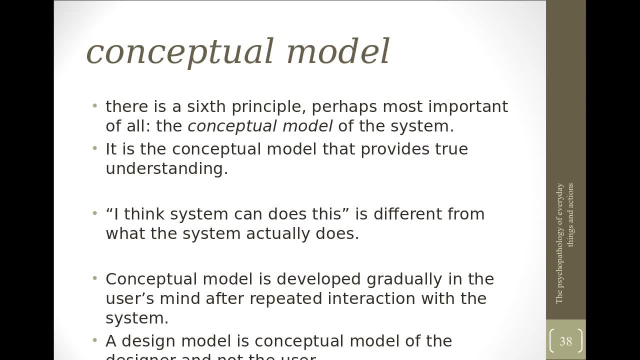 called as the conceptual model of the system. What actually is being done and what actually the user gets considers is the concept of the system. What the user considers is the conceptual model. It is a conceptual model that provides the understanding of the system, how the system 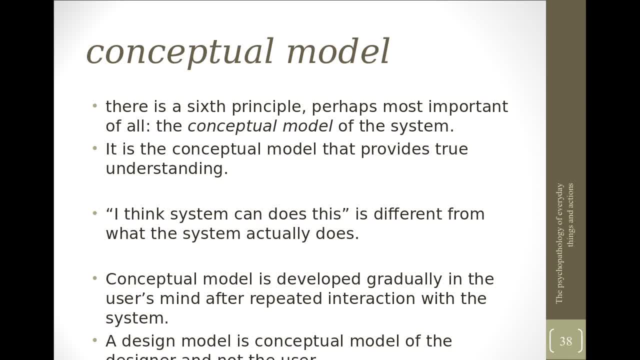 works that we know. that is what is called as the conceptual model, For example, I think the system can does this is different from what actually the system does, So conceptual model is developed gradually in the user's mind After a repeat of the process. 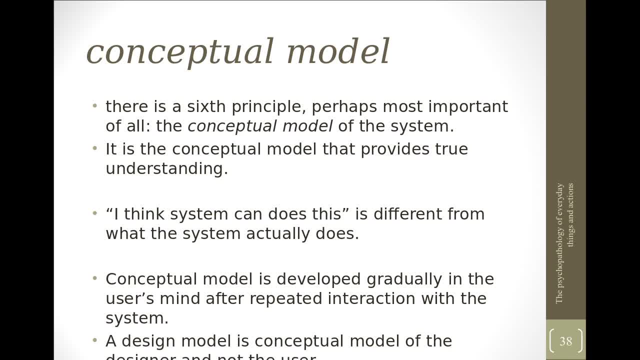 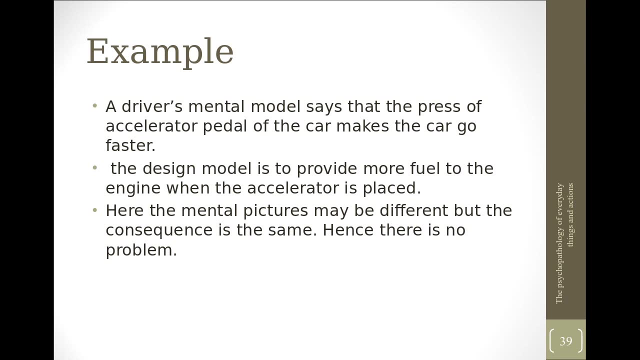 After a repeat of the process, After a repeated interaction, repeated uses of the system, A design model is conceptual model of the designer and not the user. We will see that with one example. A driver's mental model says that the press of accelerator pedal of the car makes the 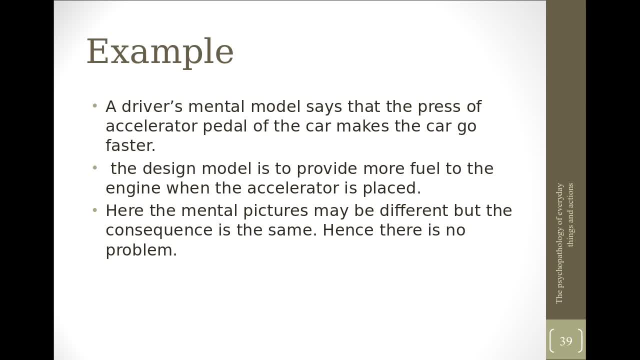 car go faster. You may not be knowing the mechanical things that we are going beneath. So how, What exact things are being done so that when we press the accelerator, the car goes faster, goes forward? Here the mental model says that when only the accelerator pedal is pressed, the car 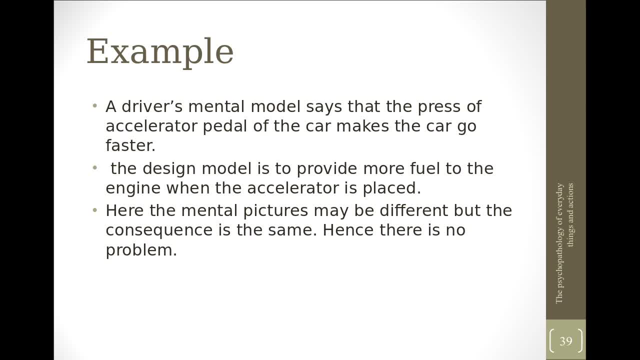 moves ahead, it goes faster, Whereas the design model is to provide more fuel to the engine when the accelerator is pressed. Here, the mental picture is like this: The car is moving forward, The car is moving forward. Here the mental picture may be different. 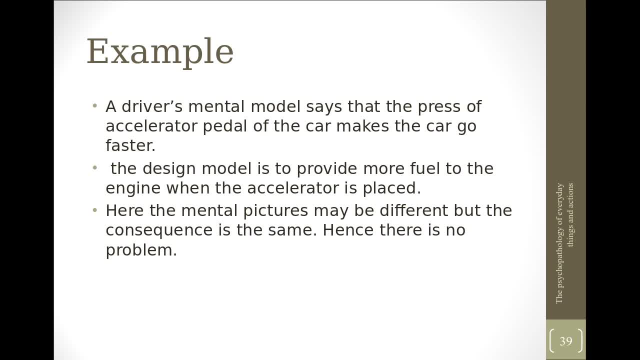 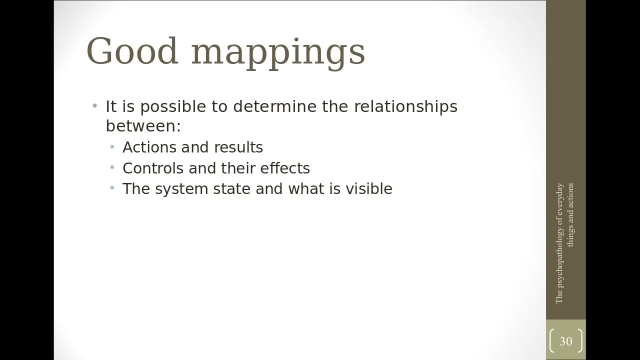 But the consequence of those two pictures or the two models is same And that's why there is no problem. So with that we will stop for today's point. Here we have seen different principles. To summarize what different principles we have seen, let us go to the first slide and